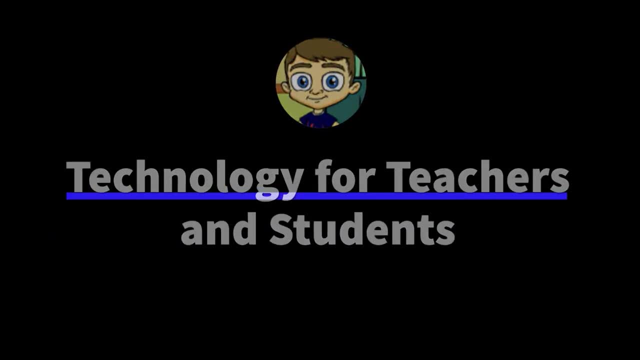 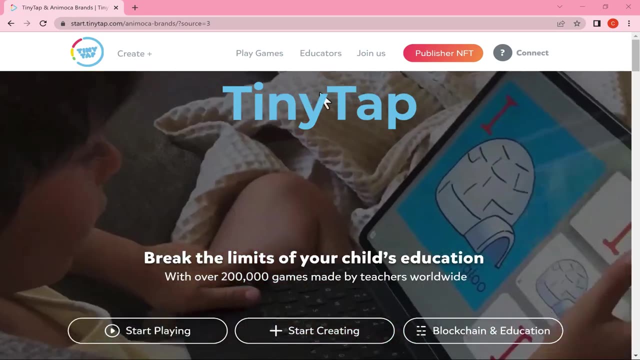 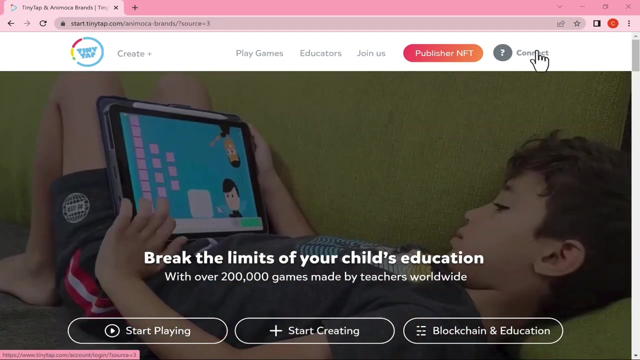 In this video, I will show you how to create your own educational games using a tool called TinyTap. Here I am on the TinyTap website and you can get there just by going to tinytapcom, and once you're there, you can just click connect. 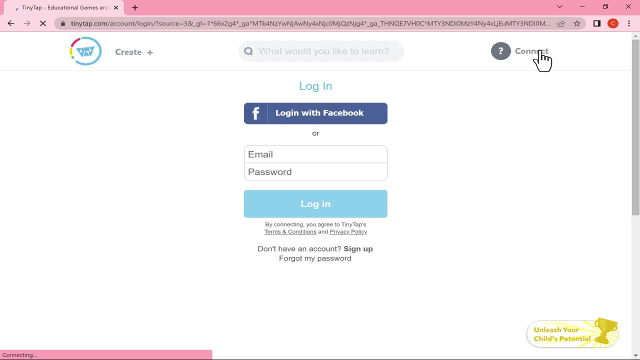 or start creating. I'll click connect and it takes me to a screen where I can log in with my Facebook account or I could sign up for a free account. If I already have a free account, I can just put in my email and password to get started. Give. 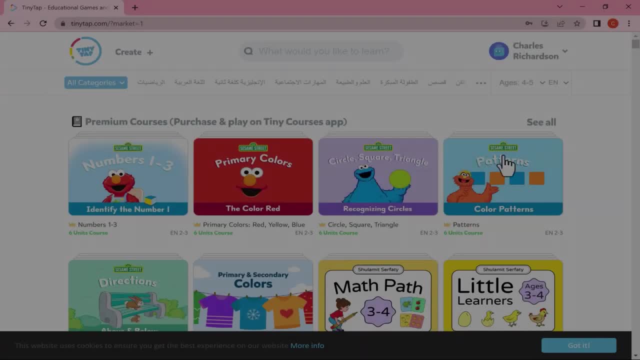 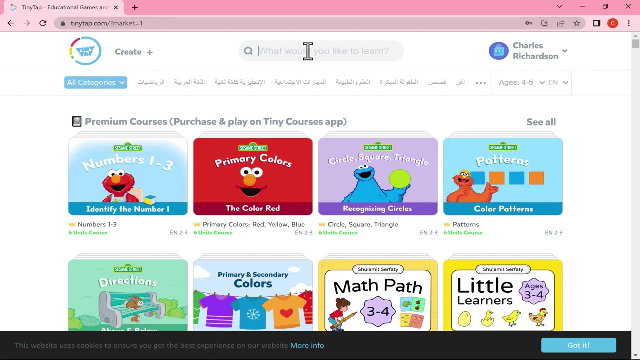 me a minute to sign into my account and then I'll resume the video. Once you're logged into your account, you'll see a few premium games and courses, and you can also just do a search for the kind of games that you want to find to make. 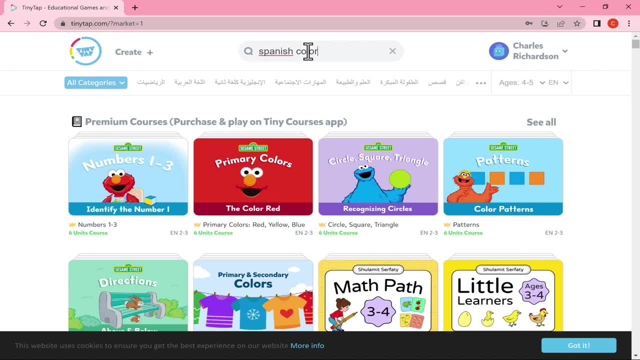 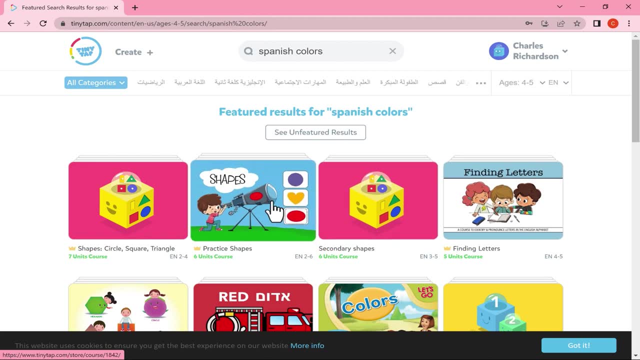 available to your students. These are games made by other people, so, for example, I'll do a search for Spanish colors, and it brings up a whole bunch of games and other activities that may or may not match what I'm looking for. So that is one way to use TinyTap, just as a way to find games and activities. 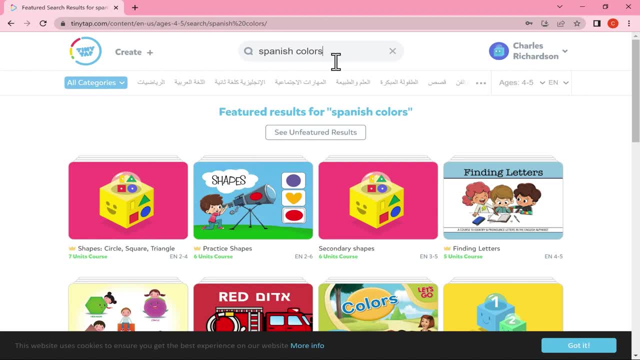 created by someone else and then using them for your own purposes. But even better than that, in my opinion, is using TinyTap to create your own games. Let's take a look. I'm gonna click here on create and it opens up this page that I 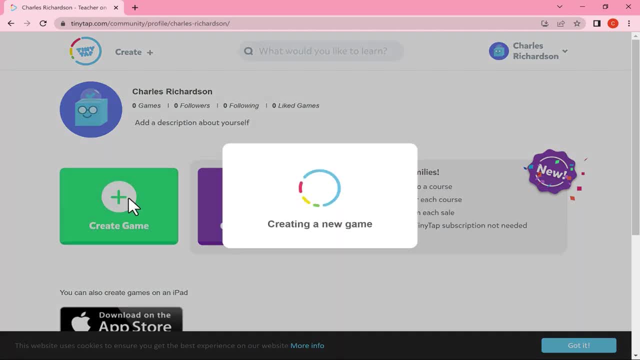 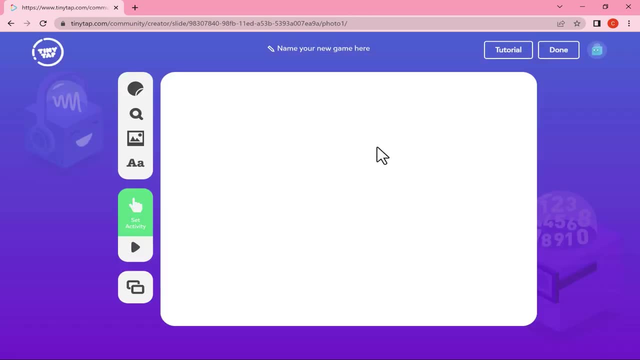 can use to create a new game. I'll click on create game and TinyTap takes me to a screen where it tries to teach me how to build using TinyTap, and that's very useful, but I'm gonna click away from it to get to the blog. 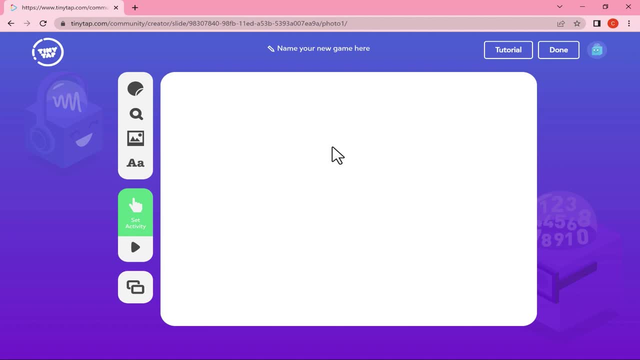 It's going to show me the blank screen on which I'm going to start creating my first TinyTap game. Before we dive in and create a simple game, let's look at the interface that we have here. In the upper left corner area of the screen, I have 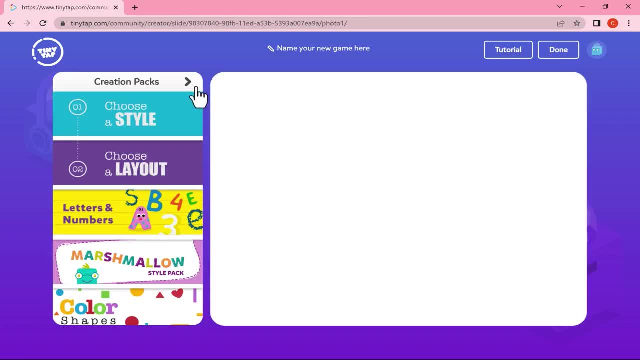 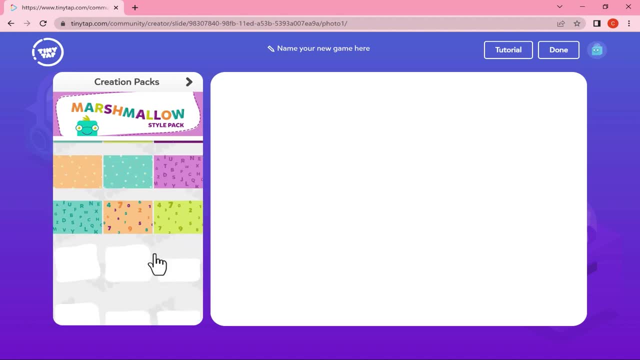 this interesting looking circle. If I click on that it takes me to a series of creation packs that I can use. You can see there's a Marshmallow creation pack that's got Marshmallow style. If I click here I can go back to the list of all. 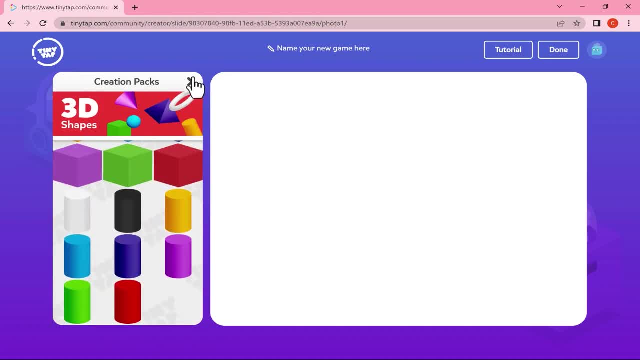 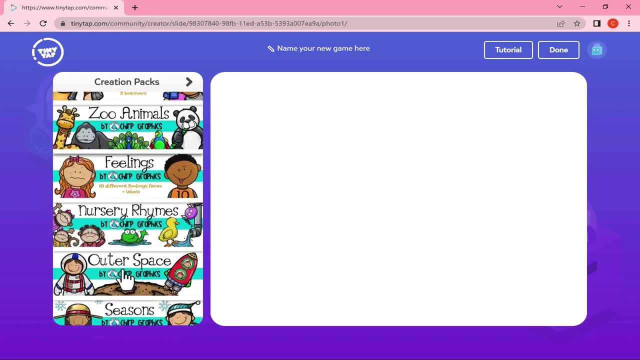 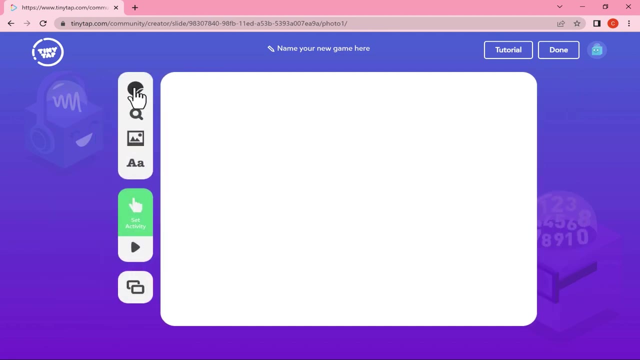 the creation packs pack with some great shapes. I'll click back. We have frames, we have diploma back to school- just a whole series of really fantastic creation packs And we're going to use one of these in just a minute. I'll click here to go back Below this button that takes us to the creation packs. we 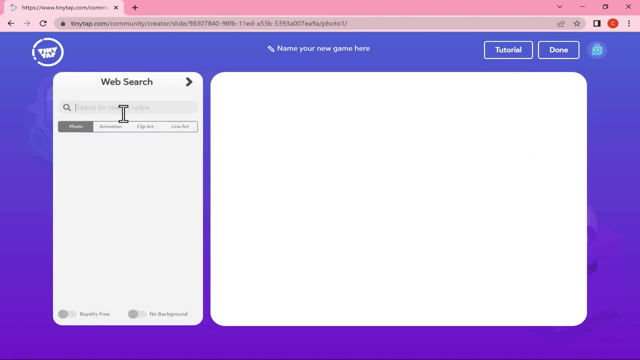 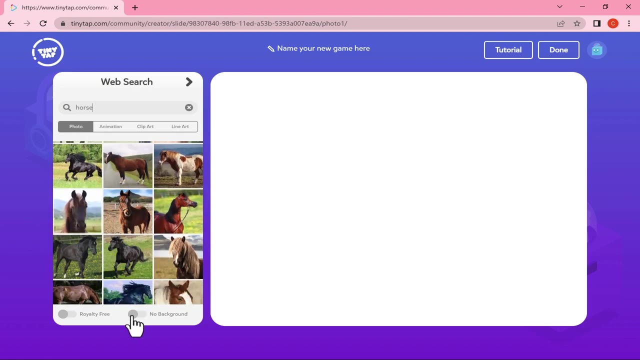 also have a magnifying glass. If you click there you can search for images, animations, clip art and line art that you can bring into your projects. So, for example, let's say I need a horse. I can do a search for horse. It brings up some great results. With a click of a button I can. 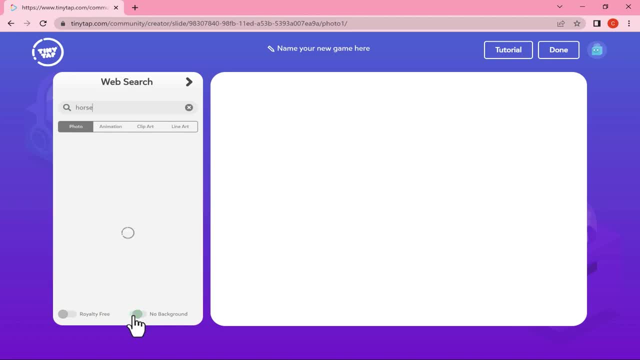 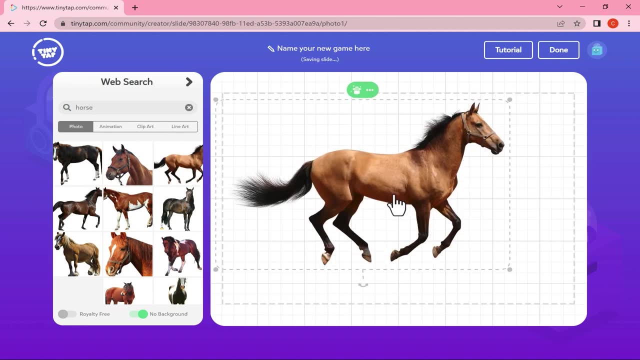 eliminate images that have backgrounds. So I'll click here and now it only shows me horses with no backgrounds, And you'll see in just a minute how important that may be to get rid of the backgrounds. You can click on any of these to add them to your project. I'm going to click on each. 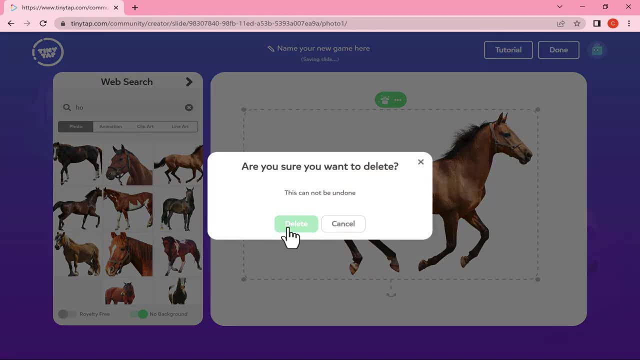 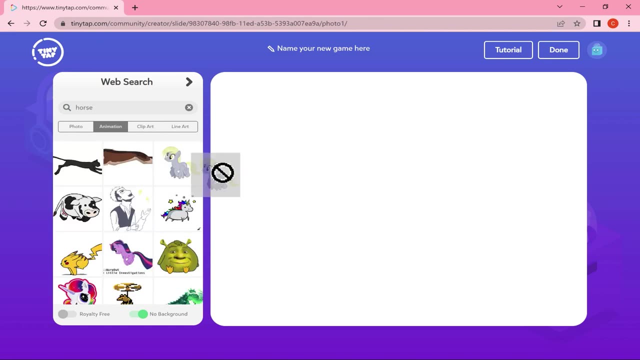 horse in turn and tap delete to remove them. I'm going to remove them from this project. Notice that I could also click here on animation to get some animations, some of which are animated horses and some may not be Clip art. there's some horse. 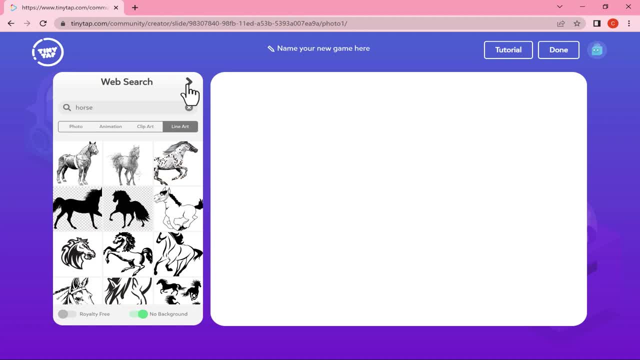 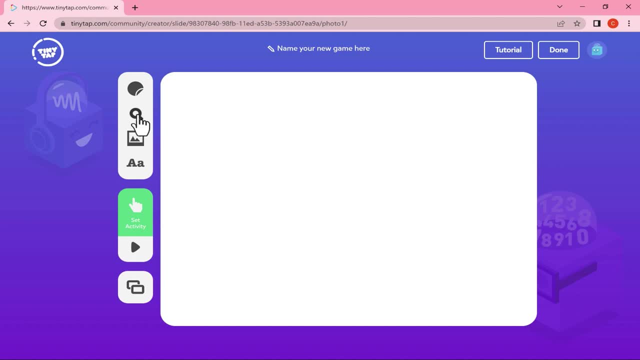 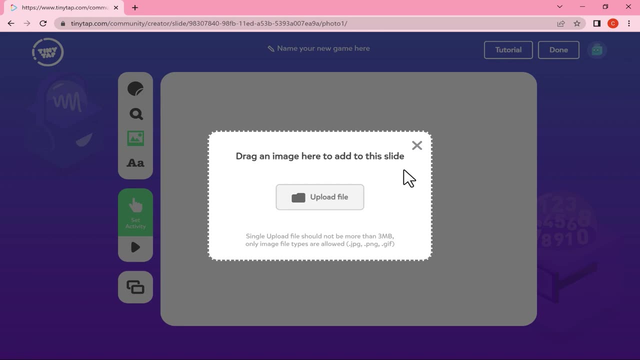 clip art and line art. I'm going to click here to go back to my project main page. Now, in addition to these creation packs and searching the internet for images that you may want to use, I do have a third button. This is for if you have an image on your computer, maybe one that you've taken with. 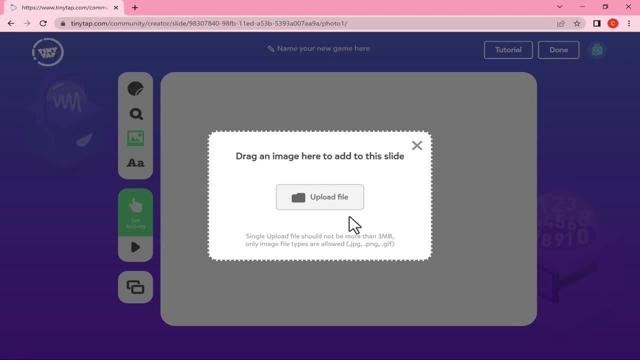 your smartphone and transferred to your computer. If you have an image on your computer- maybe one to be shown to your computer or any other image that you have on your computer- you can click to upload that file into your project. Below that we have a text box tool. If you click there you can type, and this is: 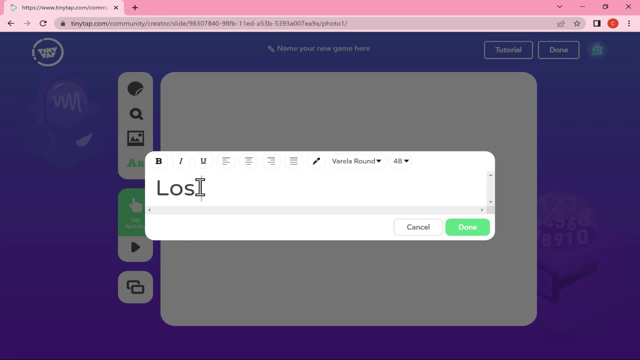 exactly what I want to do in this case. You can click and type some text that you want people to see as part of your project, So there's some text that I want to include and I've selected it. I might want to make it bold, or. 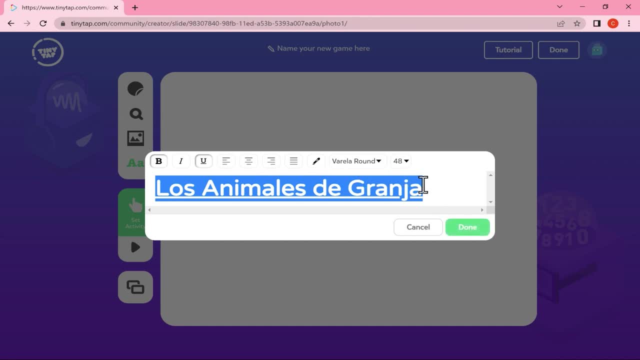 underlined. Whatever you want to do, you can see the other options here as well, But I'll just click done. There's my text and I'm going to gonna drag it up here to the top and make it bigger just by using one of. 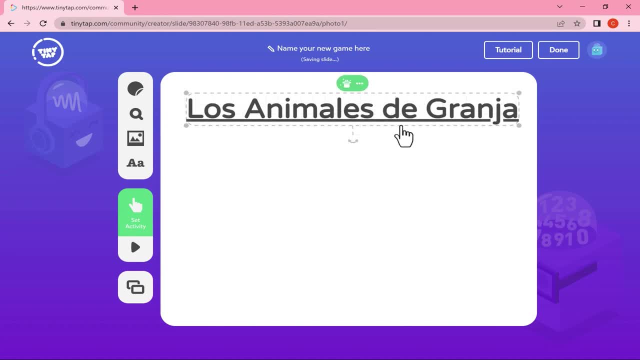 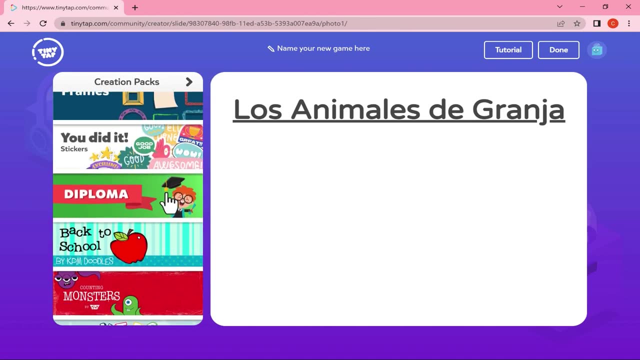 these handles in the corner of the text box and this is gonna serve as the title for my game. To go with that title, I'm gonna go back to this creation packs button and browse down, and I'm looking for farm animals. There should be a. 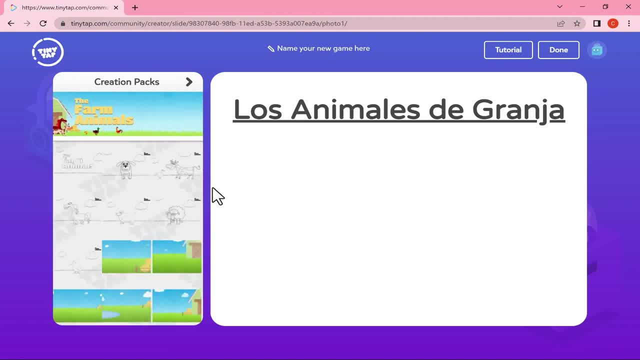 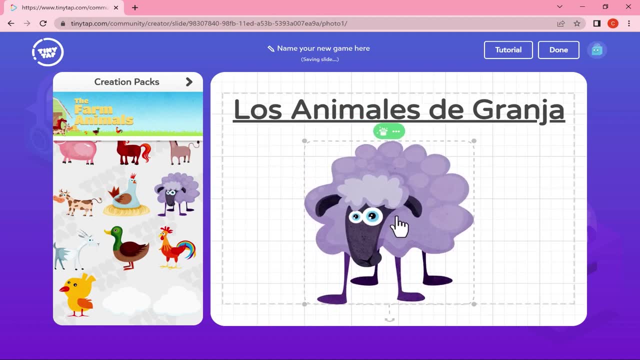 creation pack down here. yeah, here it is called the farm animals and I'm just gonna select one of those farm animals and make it bigger and this is just gonna be basically the welcome screen or the cover for my game. At this point I'm done with my first screen or level in my game, so I'm gonna click here on. 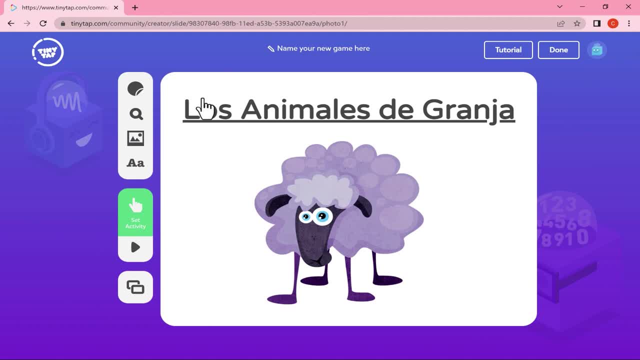 this button in the upper left to get back to the creation packs and then again to get back to this interface. Now that you know about these four buttons here in the upper left, let's move on to look at these tools and what their purposes are, and we're gonna look next at this particular button When you click. 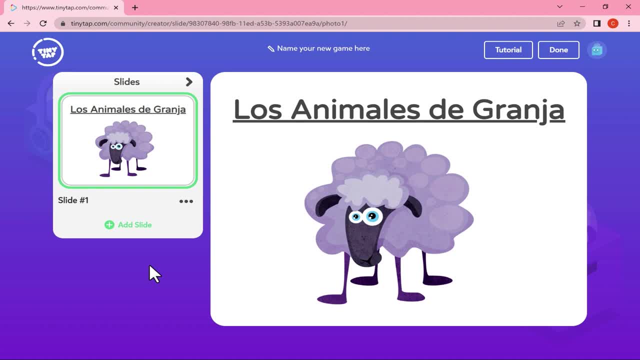 on this button. it shows you your project so far, the screens or slides or the tree. So let's move on and we're gonna click on this button and this button is gonna show you your project so far, the screens or slides or the levels that you've set up. So right now I only have one slide or level and it's my. 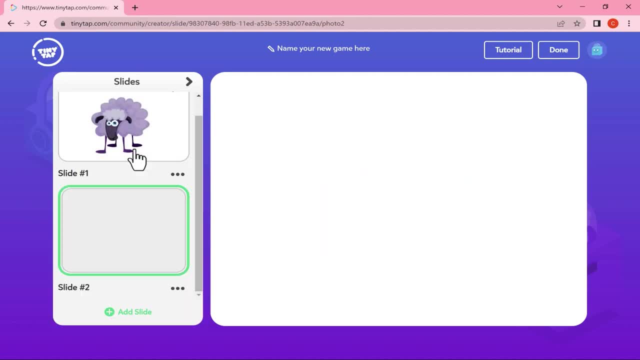 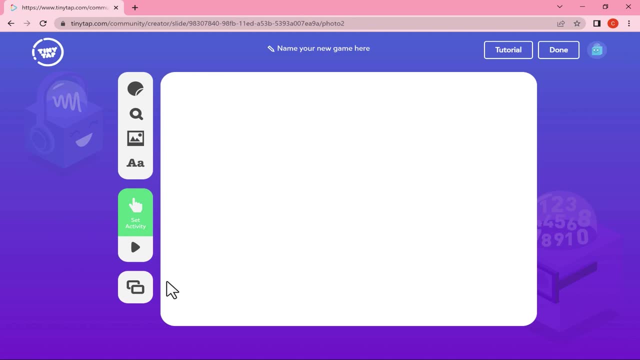 title slide. I'm gonna click here to add a second slide. Now that I've got that second slide, I'll click this button to go back to my main interface and you can see it's blank and it looks like I may have lost my work of my title slide. but 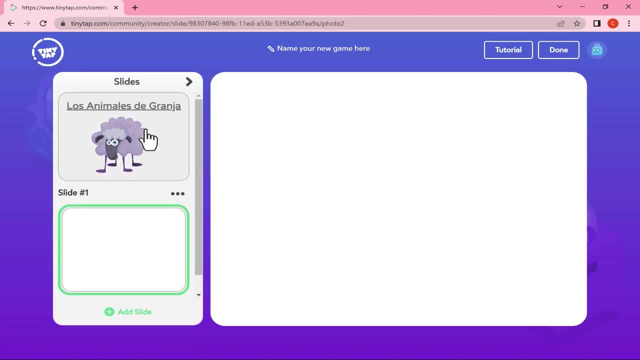 that's not the case. I can click here at any time to see that I still have my title slide here at the top. Again, I'll click here to get back and I'm gonna click here on this creation packs button to once again jump back to the 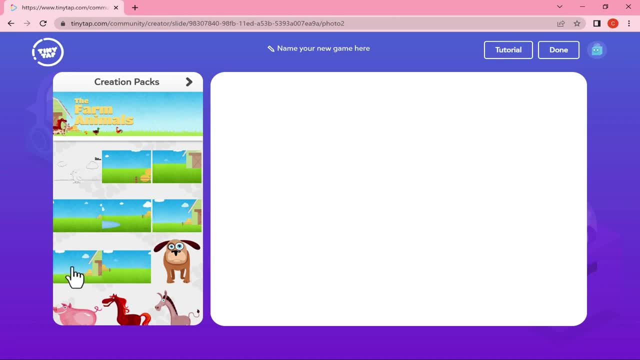 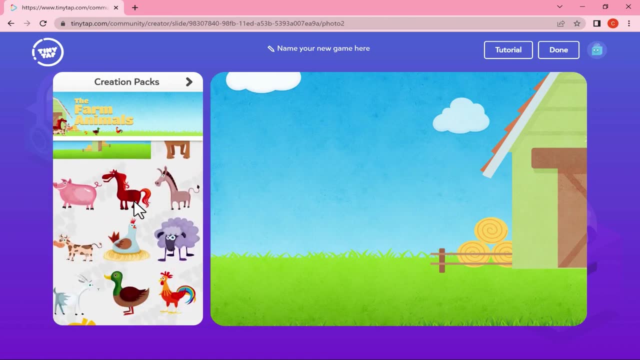 farm animals creation pack, because this time I want to use a background. I'm gonna click here to select this background, to add it to my slide or my level in my game, and then I'm going to select a few animals. How about this hen? 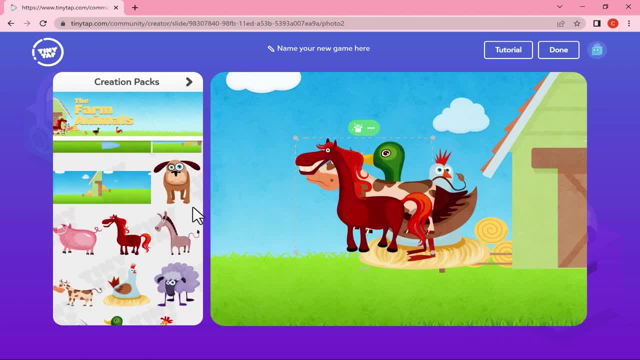 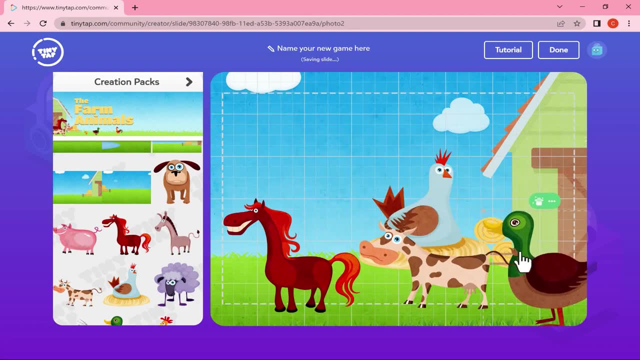 this duck, a cow and a horse. As I've been selecting these animals in the creation pack, they've been added to my slide and I can now click and drag to move them around and put them where I want them to be. Now, as you're designing your 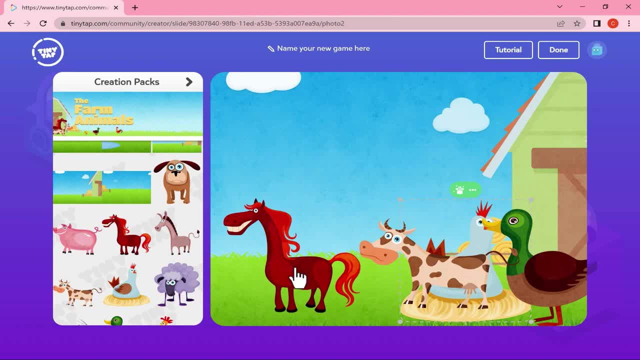 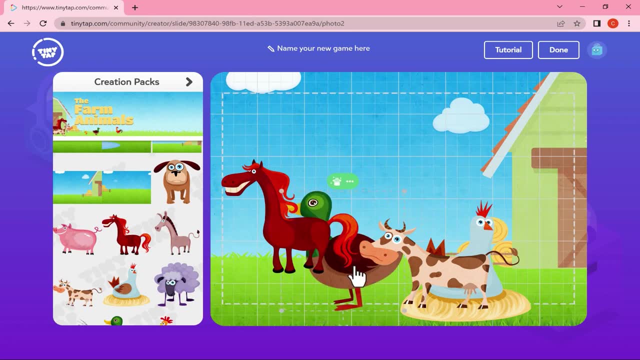 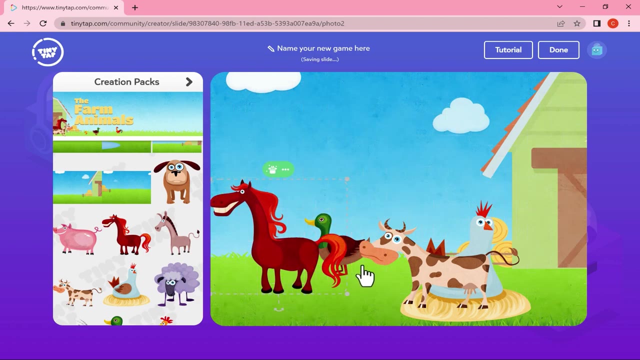 levels or your slides in TinyTap. there's some tools that you have. Yes, you can click and drag to move an object around. You can also select an object and then look in one of the corners around that object. You should see these little circular handles and you can click and drag those handles to make objects. 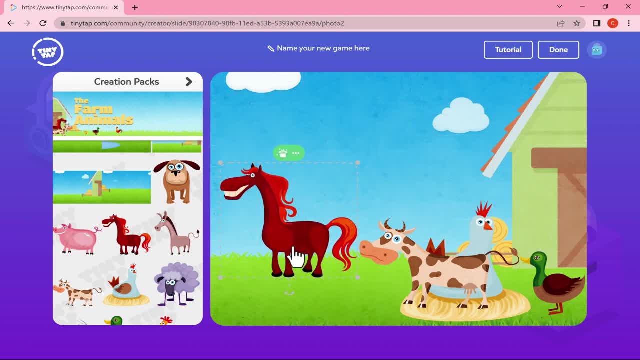 smaller or bigger. We do also have some options that appear when you right-click on an object. So I'm gonna right-click on this horse and I'm gonna move this horse to the side. I'm gonna move this horse to the notice that there's some options. You can affect. the background, you can duplicate. 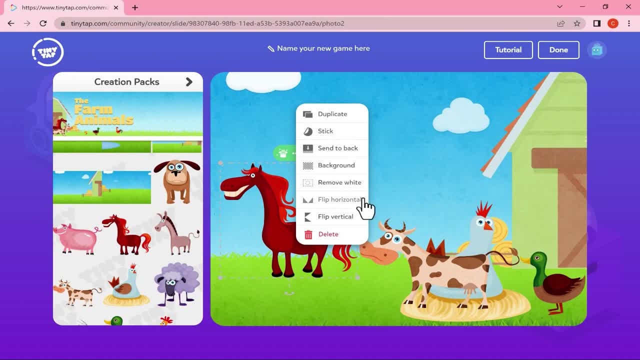 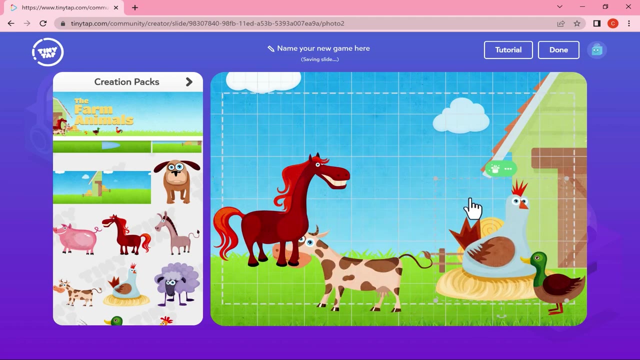 it you can remove the white color. Some of the most powerful useful features are here: Flip horizontally or vertically. So I'm gonna flip this horse horizontally. Now he's facing to the right and that will give a little variety to this scene that I'm building. So I'm gonna move the cow over here, make the cow bigger, Maybe. 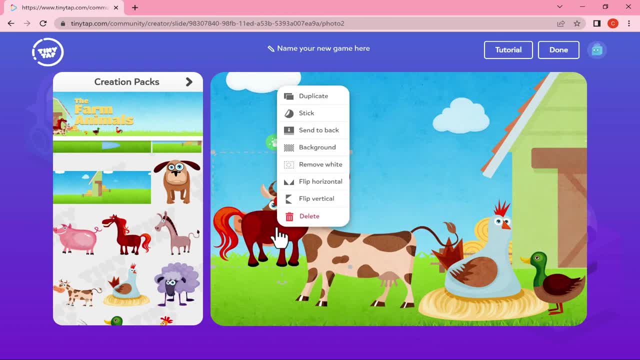 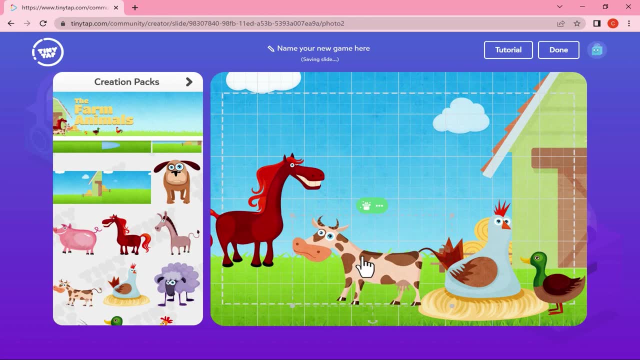 I want the cow to be in front of the horse, So I'll right-click on the horse and choose send to back. Now the horse is behind the cow, So those are some features that you can practice with. I'm gonna make the hen quite a bit smaller. 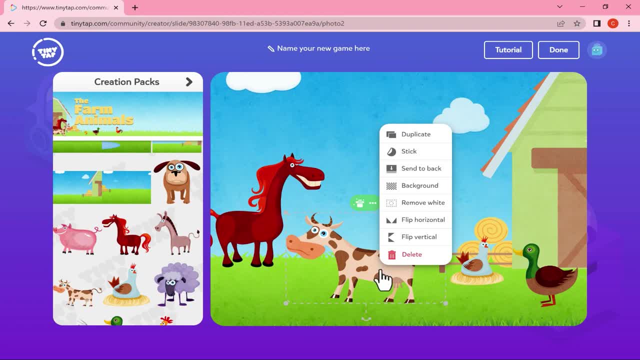 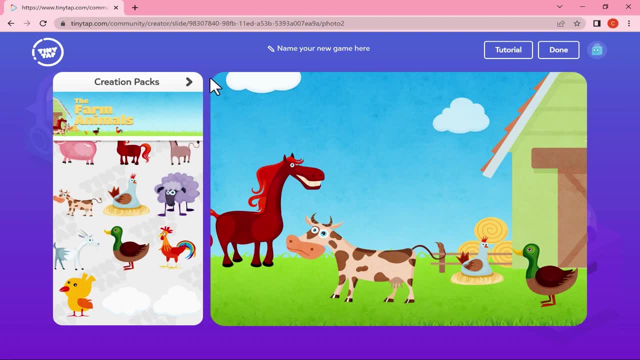 So definitely try out those tools that you get when you right-click on an object. At this point, I want to get back to the main interface and I could click the arrow here in the upper left, like I've done in the past, or there's a. 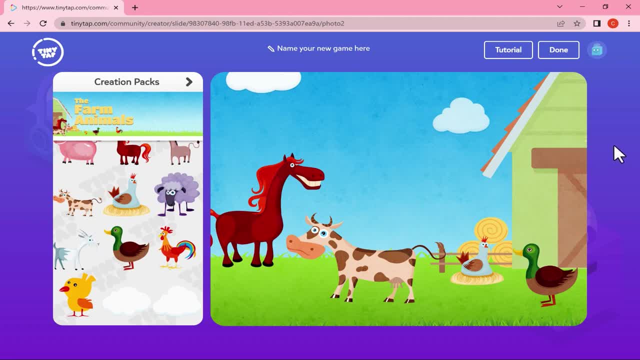 shortcut. If you just click away from the slide or the level that you're building, it takes you back to the main interface. Okay, so now we've looked at these four tools, Now we're going to go back to the main interface and we're going to click. 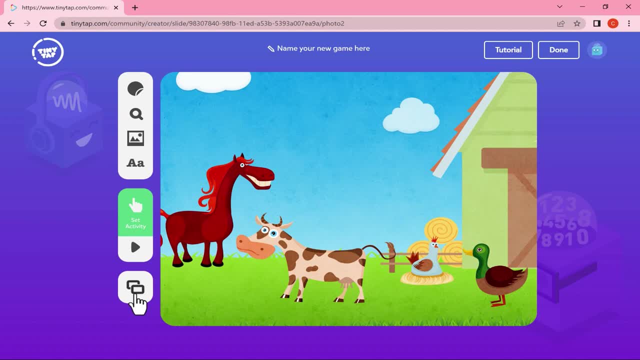 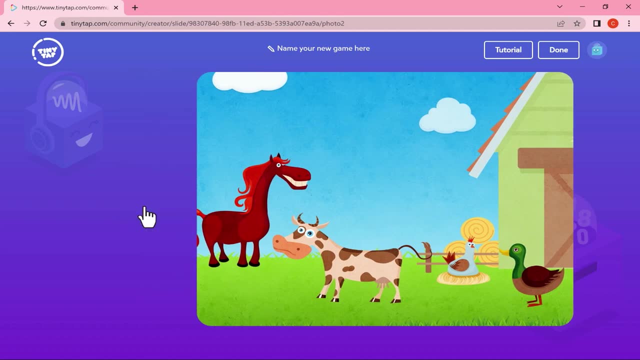 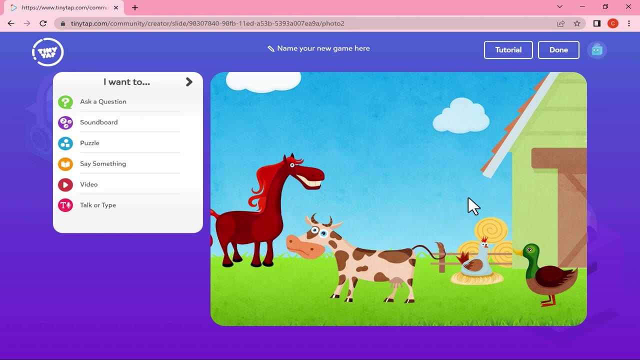 on the set tools. We've looked at the slides tool. Now we get to actually build interactive activities into this game. So I'm gonna click here on the set activity button and this brings up six different activity types that I can apply to this slide or level in my game. In my case, I want this level to be all. 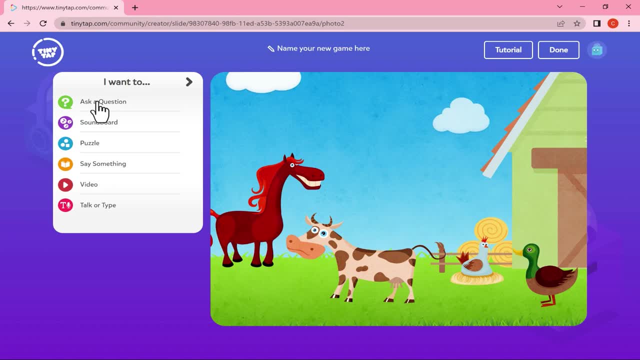 about asking questions and answering questions. So I'll select that option and then I'll record my question. So I'll click record question. TinyTap wants to access my microphone. I'll say allow by clicking here and then I'll record my first question: Donde esta el pato? When I was done recording, I clicked stop and 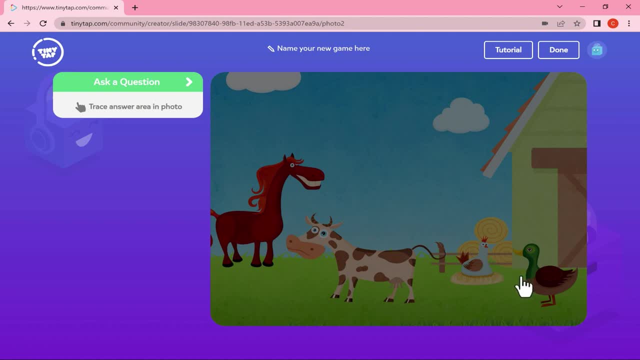 now all I have to do is draw a circle around the correct answer. So el pato means the duck, So I'm just clicking and dragging to draw around the duck in this slide. So there's the duck Now. when I release the mouse button it turned my 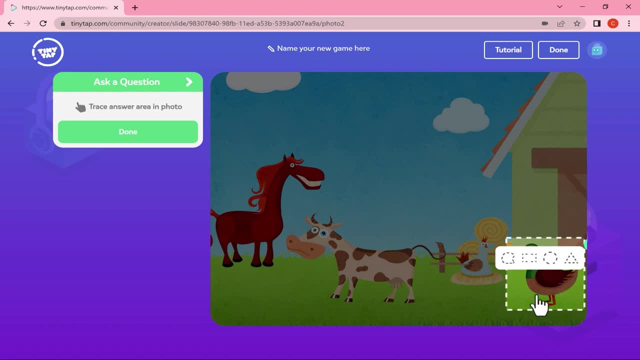 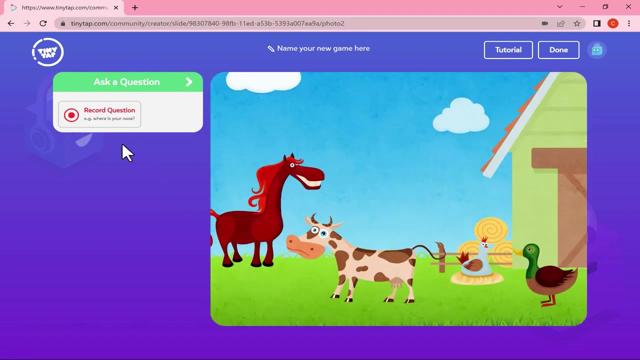 very careful outline into just a square. If I prefer to keep the precise outline that I drew, I can click here to go back to the precision outline and then just click the check mark. and now I have question one recorded and the correct answer outlined. Now I can add a second question by clicking here and 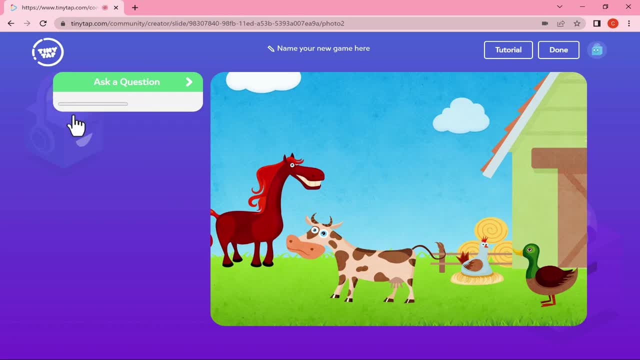 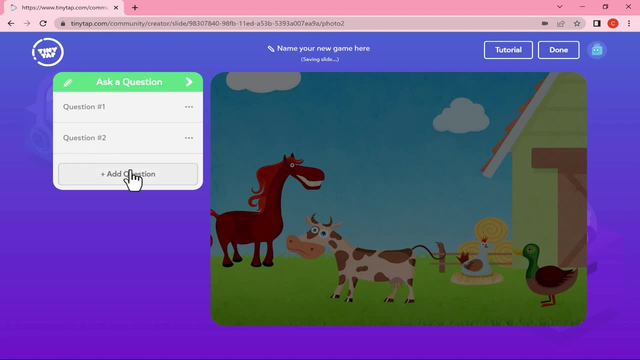 clicking record question: Donde esta la vaca- Stop, and then I can outline the cow in this case, and I'll go with the precision outline check mark. There's question two. question three: record question: Donde esta la gallina? Stop, and then I'll. 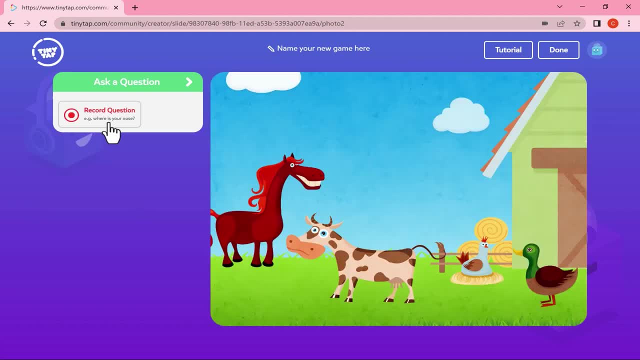 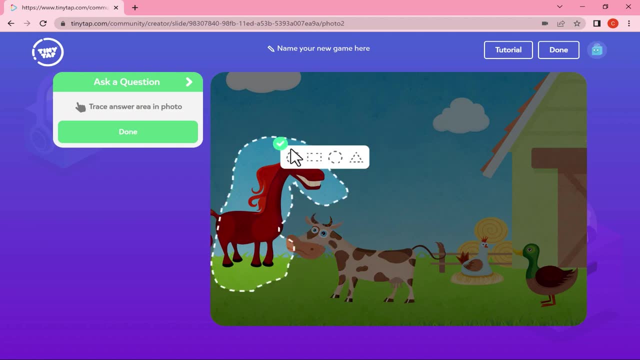 draw an outline around the hen. Click there. and my final question: Donde esta el caballo? And I'll outline the horse. So pretty quickly I've been able to add four questions and four correct answers in to this game. At this point I could. 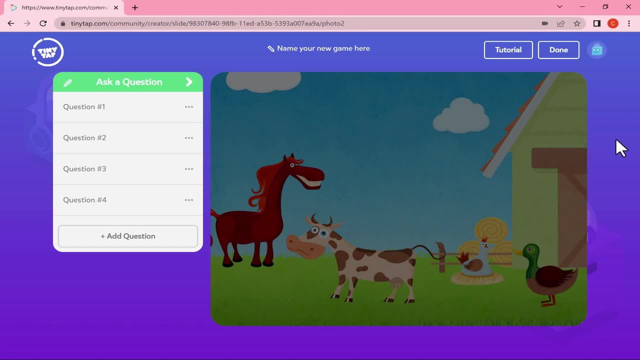 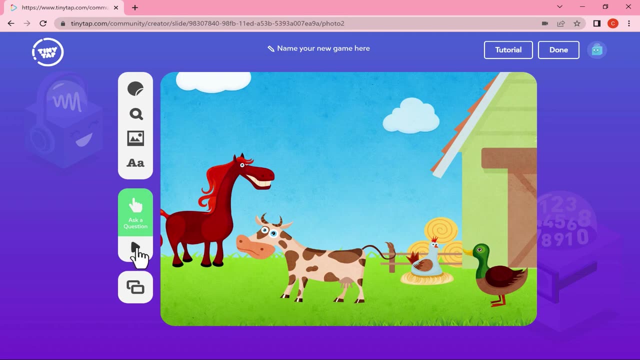 click these arrows to get back, or I could just click away from the slide or the level, and it takes me back. Now let's look at the final button that we have here as we're building our project, and that's the play button. So I'll click play. It takes me to the level. 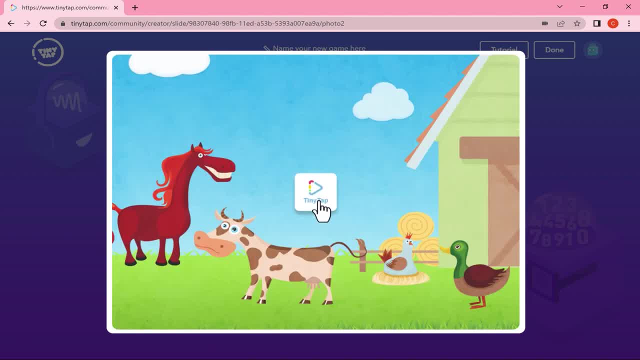 where I've submitted all thewon functional. So let's continue and you can write down the names and things that Iηve gotten level I'm working on and I can click the tiny tap button to play it. So there's my question, Here's the answer, so I'll click there. I got it right. Next, 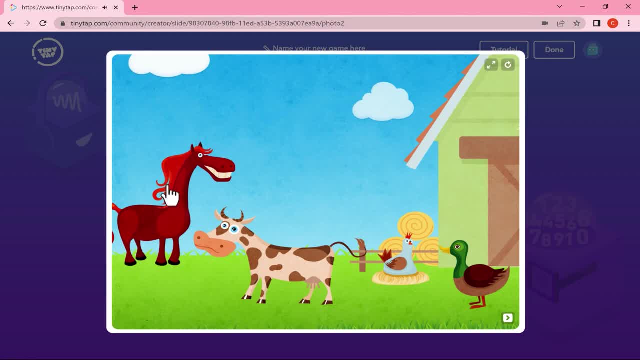 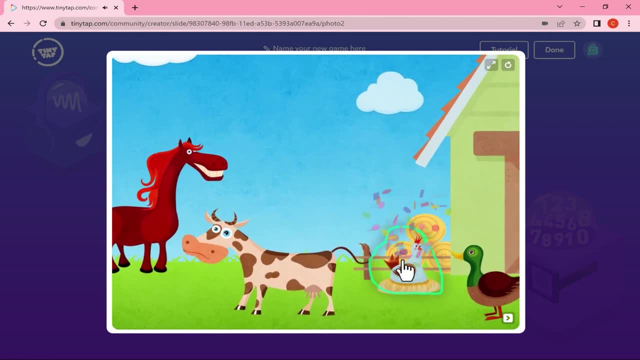 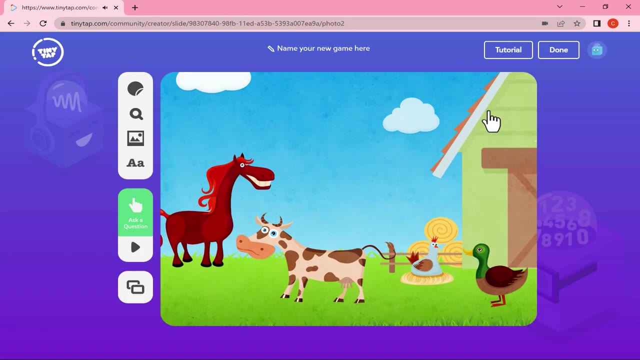 question. This is the correct answer, but I'm gonna click on a wrong answer and then back on it and then back on the right answer, and so you can see my game is working very well so far, and now that I finished the activity it takes me back to the editor, So my game is coming together very well. 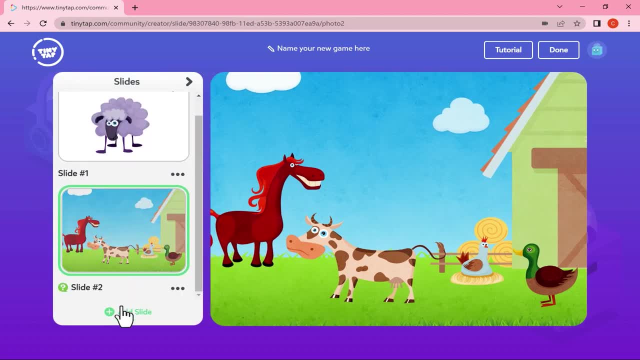 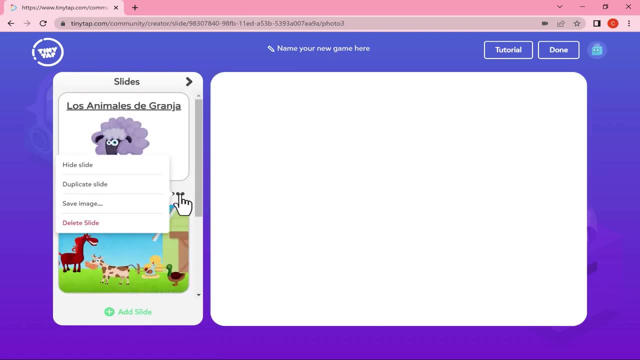 At this point I could click here on the slides button to add a third slide, a fourth slide, whatever I want to do. I can also click on a particular slide using these three dots and then choose to duplicate a slide, and then I could make. 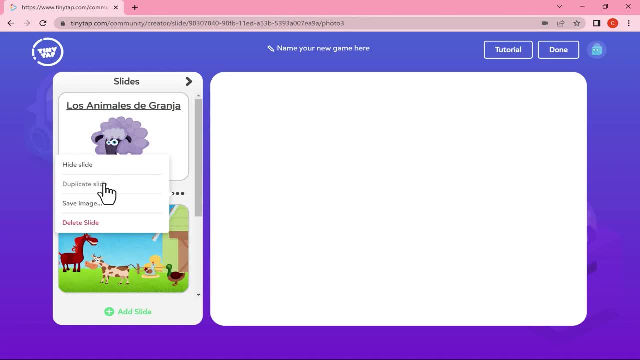 some slide adjustments: maybe move the animals around, make them smaller or bigger, change the animals on the second slide. There's lots of good things that can happen when you duplicate a slide and then change some of the features of the slide. It's a great way to come up with a second level or third level very quickly. 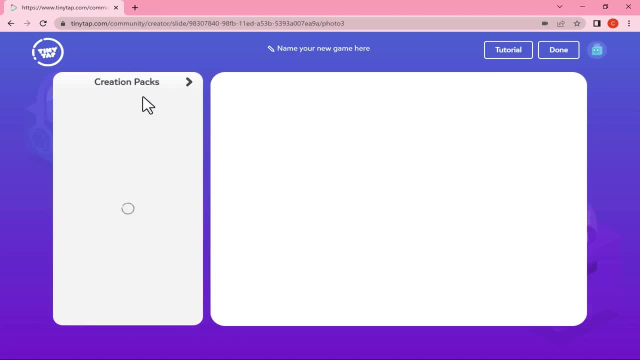 In this case though, let's say for this third slide, I would like to try a different type of activity. So, going back to the farm animals, I'm gonna choose a different background and maybe a few different animals, and now that I've chosen those animals, I can click away from the creation pack and from the 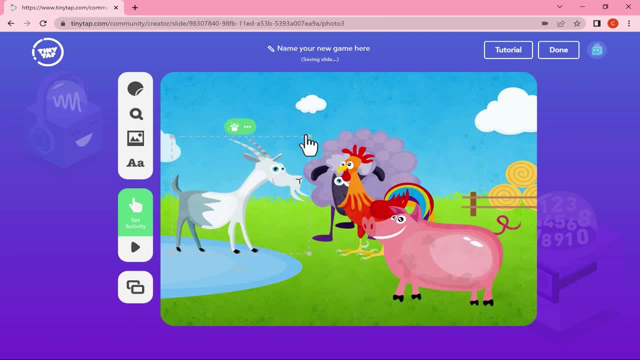 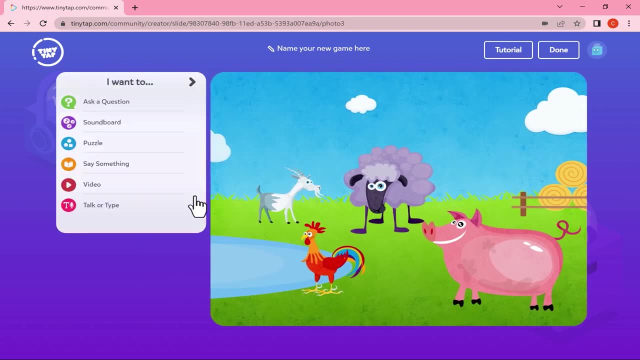 slide to get back to the main interface and I can organize these animals and place them on the screen in the places where I want them to be. and for this new slide I want to set a different activity. So, as you're building your games in TinyTap, you could build a game that features only ask a question. slides. 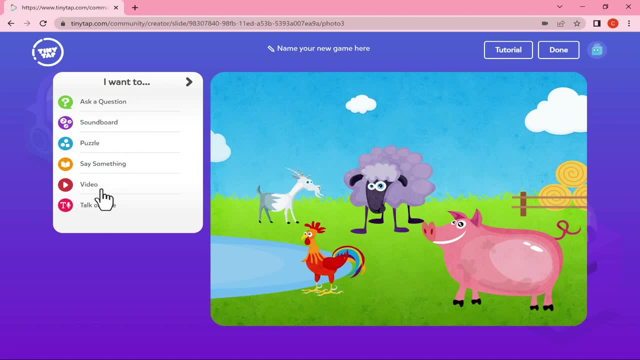 That's all that it's made up of, or you could mix it up. You could have one level that simply says something. This may not be really considered to be a game feature, but basically on this slide I could just record a message that I want. 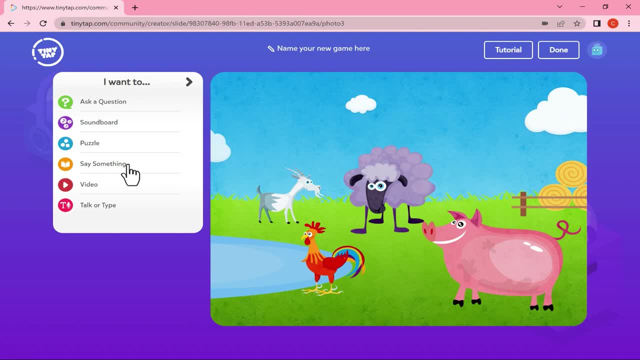 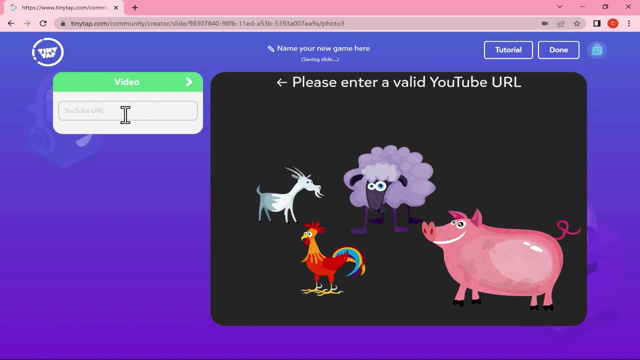 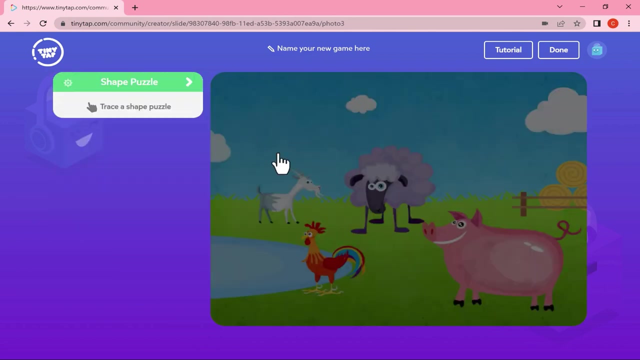 the audience to hear. So this is great for creating narrated books or stories. I could also simply add a video video. If I click on video, you can see. you just put in a URL from a YouTube video and that video should be embedded onto the slide. I could also turn this into a puzzle just by tracing a shape. 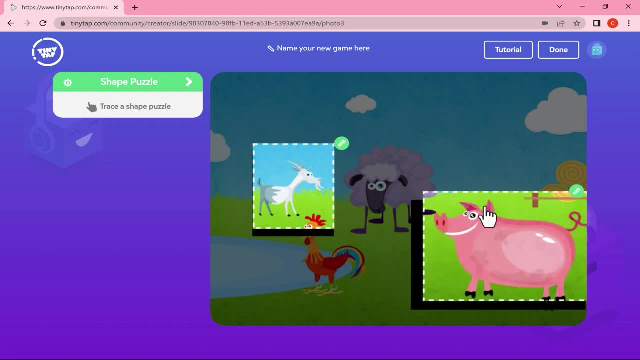 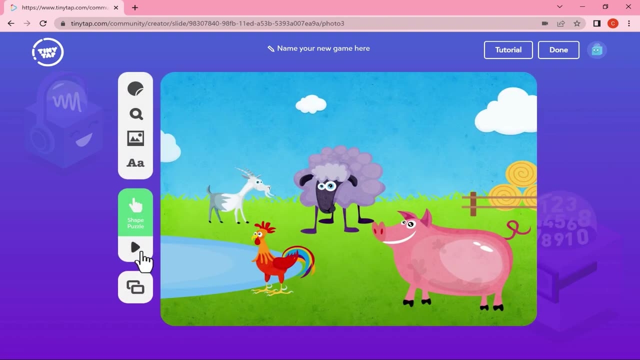 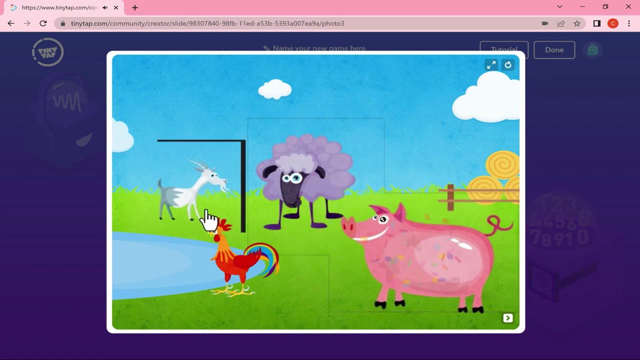 and then clicking the check mark, tracing another shape check mark, and it's basically just cutting out these shapes as if this were a puzzle. Now, if I click away and try this level or slide, you'll see the result. You have to put these things in the right places and to make this, 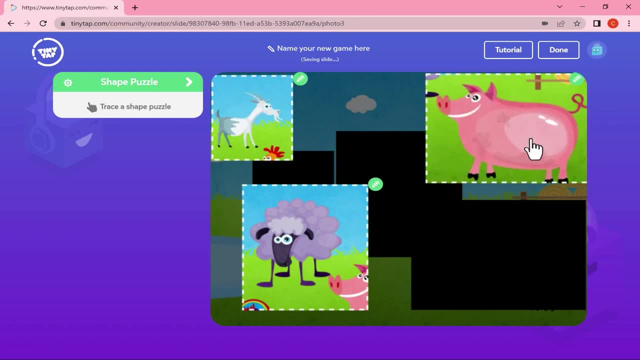 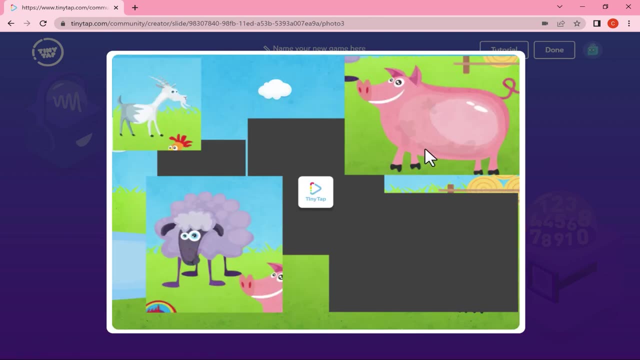 harder, I could pull these pieces further away from their actual destinations. Now, when I try the game by clicking play, you'll see that the puzzle pieces are further away from where they're supposed to go, making it a little harder. So that's another interactive feature that I can. 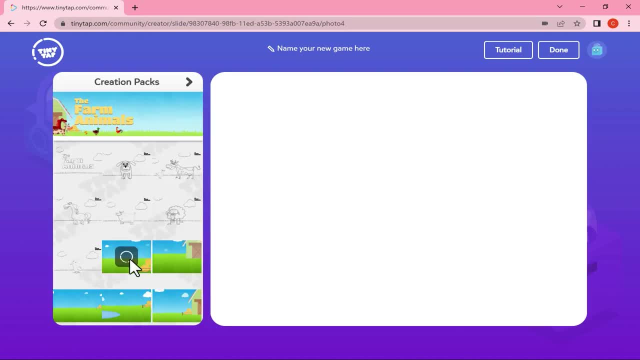 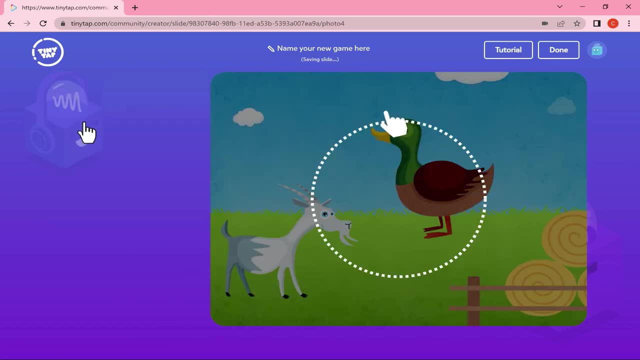 put into my games. I'm going to create one final slide just to point out that we also have a few other apps that I can use to create a puzzle. I'm going to create a puzzle that I can use to activity sets that we can try. We can create a sound board, which is pretty exciting, You would. 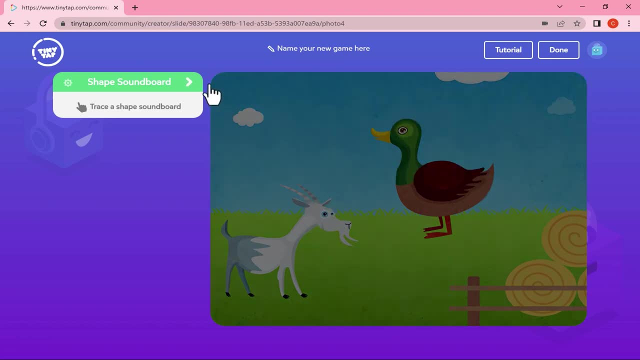 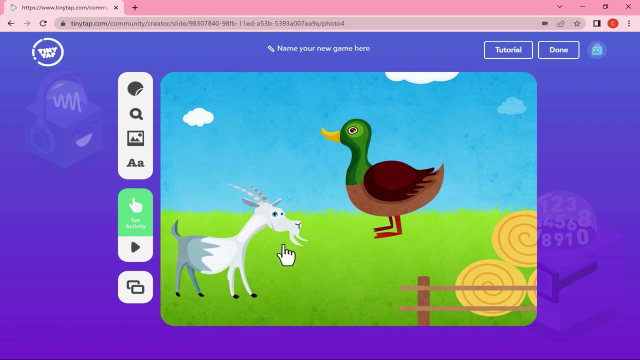 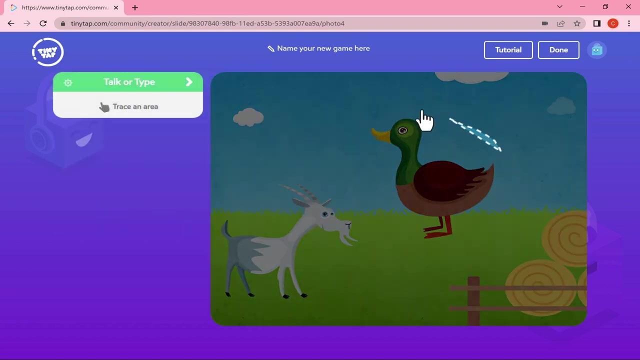 just trace around objects or shapes and anytime someone clicks on that shape or object, a sound would be played, A sound that you record, that you choose to link to that shape or object, And then, finally, we have talk or type, which is a very exciting feature. You would start by tracing an. 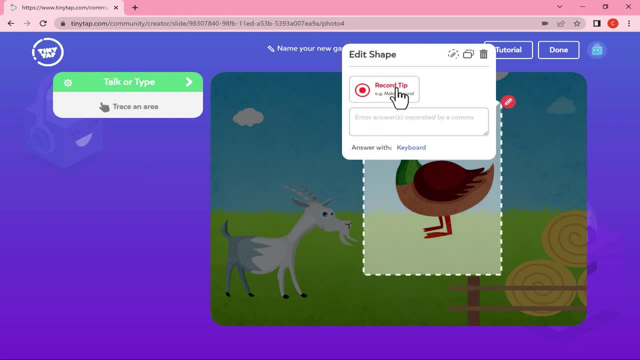 area, clicking the check mark, and then you could record a tip or a question and then type the correct answer here. You can have more than one correct answer if you want, as long as you separate it by a comma. In this case, I'll type El Pato as the correct answer. 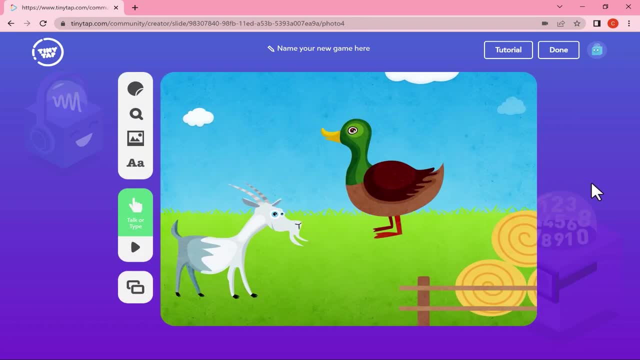 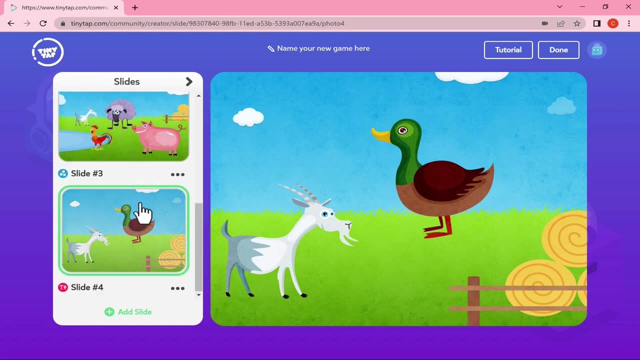 I'll click away, and if I click away from this slide completely, it takes me back to my screen. At this point I have a game with a title slide, welcome screen, and I've got three levels. I'm going to click done in the upper right corner and now I have the opportunity to publish my game. 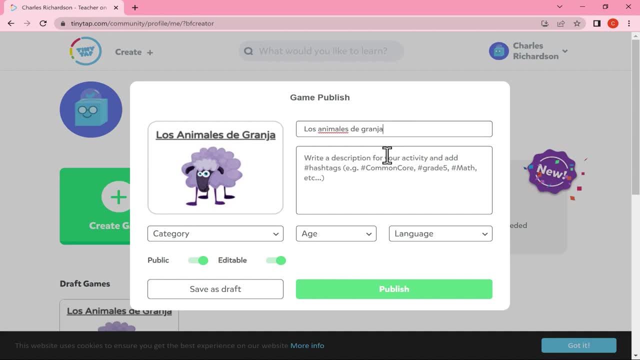 I need to give it a name. I'll just call it the same as my game name. I'm going to give it a name. my title slide. write a description, choose a category, choose a language and the age that this is built for. I can choose whether or not to make this game public for others to play If I want. 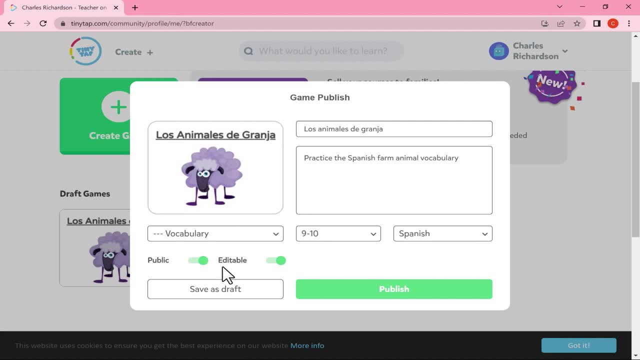 my students to be able to find and play this game easily. it's important to make it public, And then do I want it to be editable by other teachers? It's up to you to decide and then just click publish, and TinyTap is now working to publish this game so that it's visible and playable by 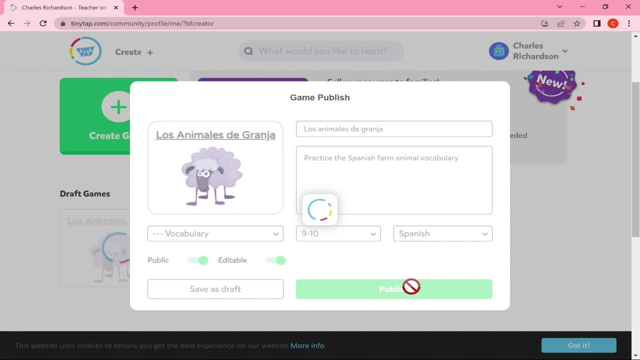 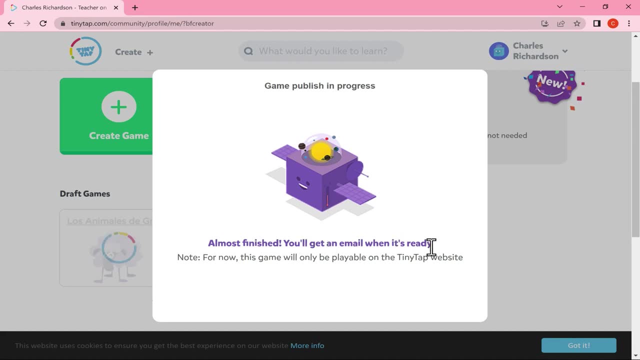 anyone on the internet. I'm going to give TinyTap a minute to finish publishing and then I'll resume the video. Okay, TinyTap has given me this pop-up that says it's almost finished. I'll get an email when it's. 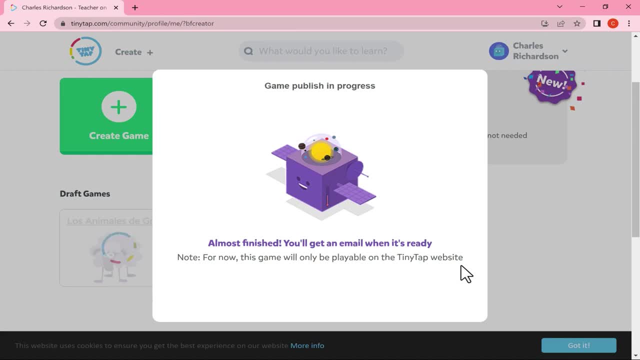 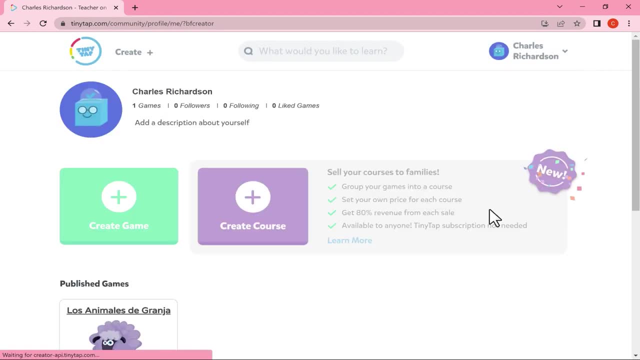 completely published, but for now the game is only playable online on the TinyTap website, not in the TinyTap app for iPad. That's okay, so I'll click away, and now you can see I have in my account a published game. Let's now look at how easy it is to make our new game available for. 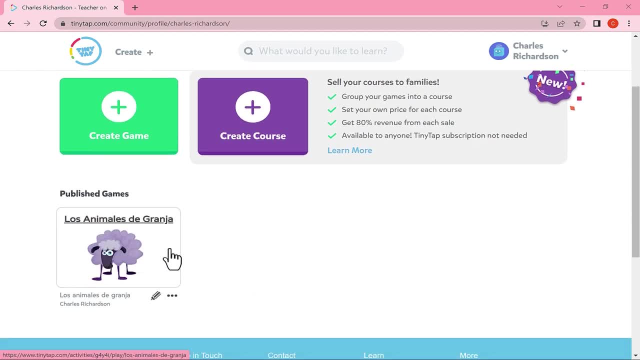 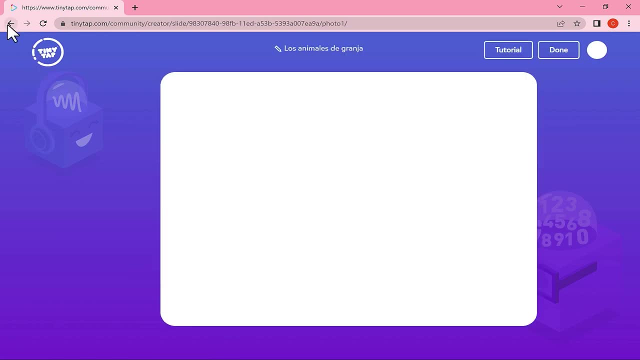 others to play. Down here below the thumbnail image for my game, I'm going to click publish. I have a couple of buttons. I have an edit button that gets me back into edit mode and I can work on the game some more if I need to. I'll click back Next to that edit button. we have these: 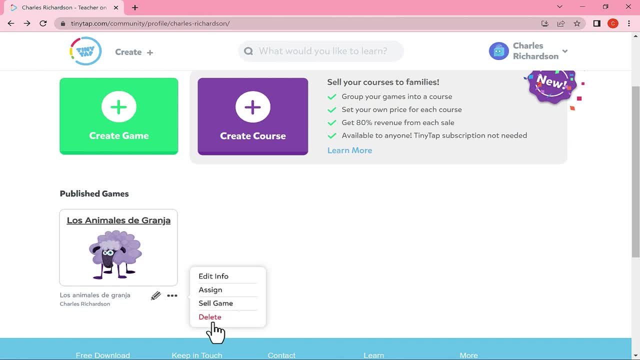 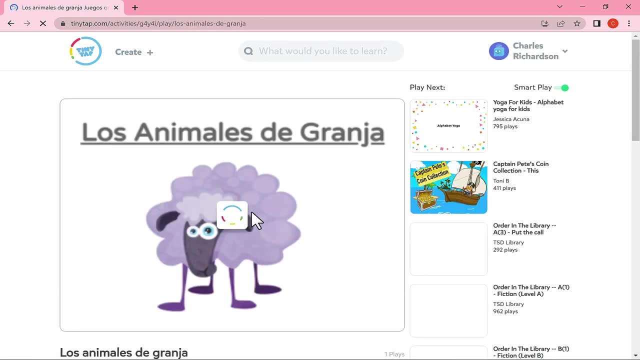 three dots, and if you click on those three dots there is an option to delete the game or to assign it to a group of students. but there's a very simple way to make this game accessible by anyone on the internet. If you just click on the game, it opens up and here the game is playable. We 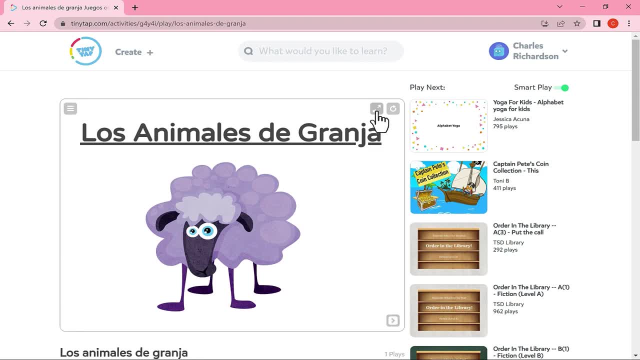 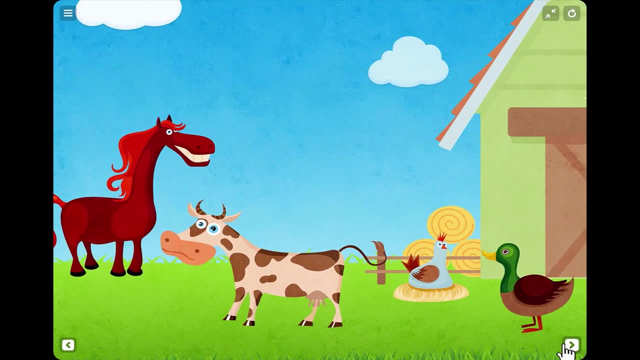 can click through and play the game. We can even make it go full screen by clicking this button here. Here in the lower right is my button to advance the slide or the level. so I'll click that. Here's level one. Here's the duck and I'll advance to the next one. Here's. 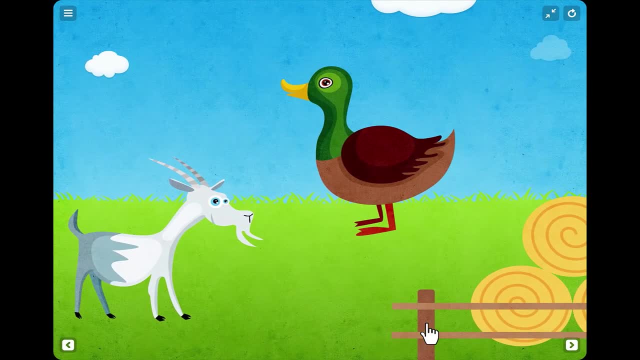 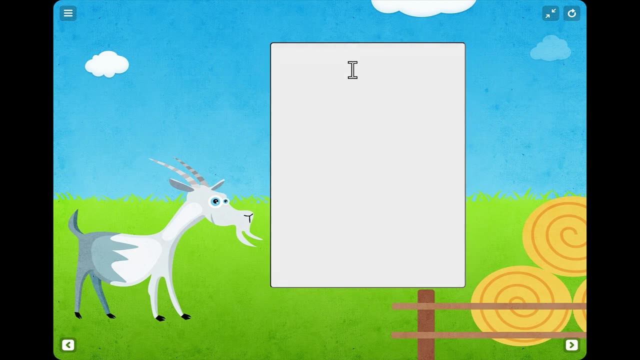 my puzzle that I can complete. Let's advance to the next slide, and here you're going to see a mistake that I made With the talk or type activity. instead of outlining a box around the duck, I should have just outlined a space above the duck, or to the right or below the duck, because what this?